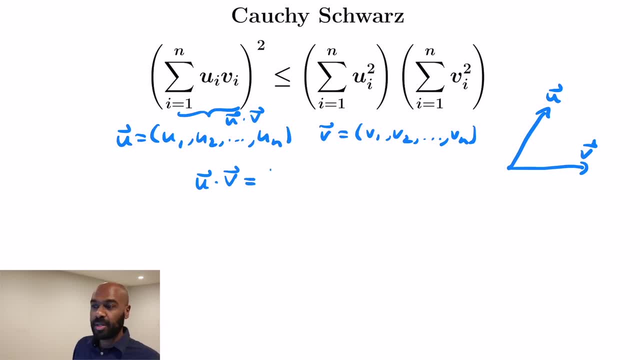 Now there's a relationship between the dot product of u and v and the length of the vectors u and v. That relationship is that u dot v is the length of u, that's the double bars. that stands for length times the length of v times the cosine of the angle between the two vectors. 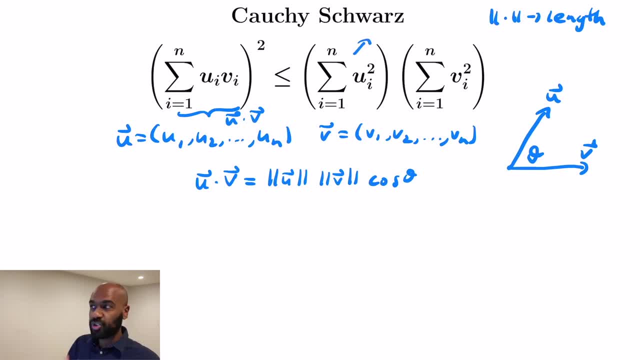 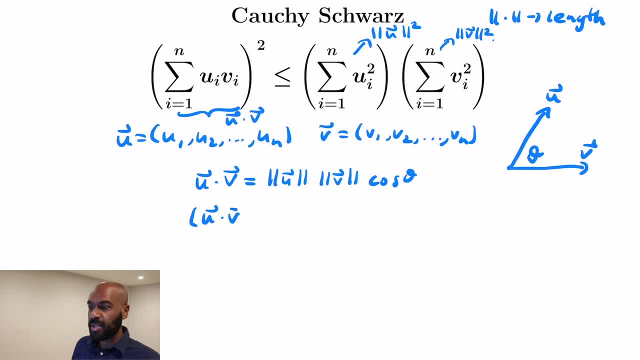 sum of the squares of the vi's is the square of the length of v. So if we square both sides in our equality here we have that u dot, v squared is the length of u squared times the length of v squared times the cosine of theta squared. Okay, and this has all the parts of the inequality that. 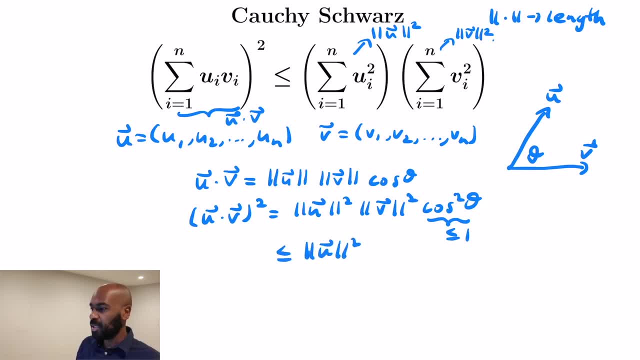 we have and we know cosine, theta squared in general is going to be less than or equal to one. so this quantity here is bounded above by the square of the length of u times the square of the length of v. The left hand side here is precisely the left hand side of Cauchy-Schwarz. 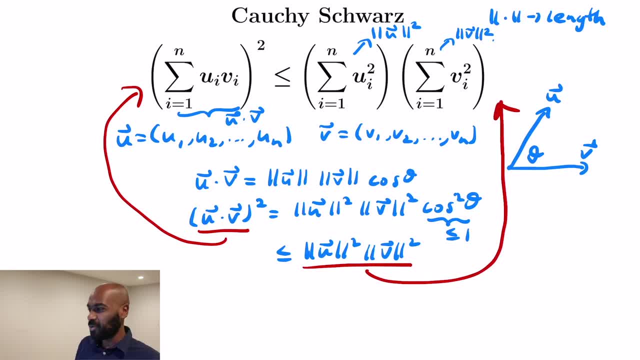 and the right hand side is the right hand side of Cauchy-Schwarz. so a great reason why this inequality holds. Now, why does equality, or when does equality hold? So, if we look at the actual inequality, equality is going to hold when cosine theta is positive or negative one. that should say: 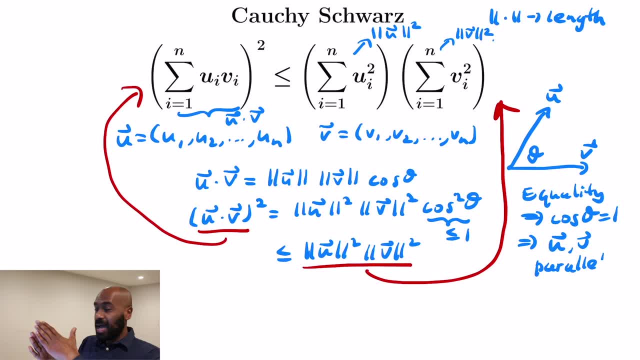 Now that means that the inequality is going to hold when cosine theta is positive or negative, one that should say: So the angle theta is either zero or 180 degrees. so u and v are parallel vectors, right? so in other words, the ui's are all the same scalar multiple of the vi's, or vice versa. So let's look at an. 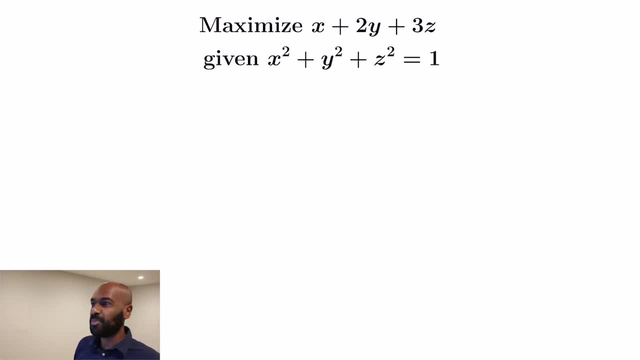 application. Let's maximize x plus 2y plus 3z, given that x squared plus y squared plus z squared is one. That's a great problem. we're maximizing a linear function subject to being on the surface of a sphere. So if we look at the thing we're trying to maximize, we can represent it as a dot product of two things. 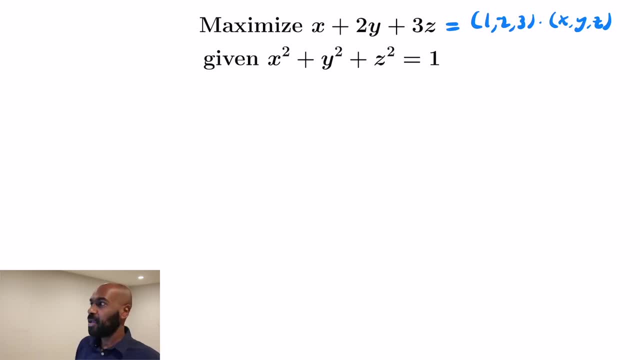 the vector 1,, 2,, 3 and the vector x, y, z. Okay, that's perfect, because then we're set up for using a Cauchy-Schwarz inequality type thing If we let u be the vector 1,, 2,, 3 and v be the vectors x, y, z. 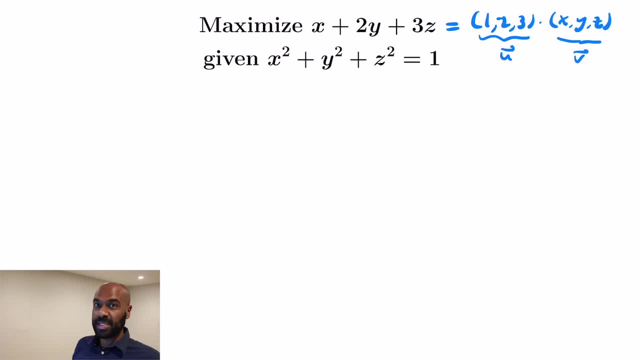 then, using Cauchy-Schwarz, we'll be able to get an upper bound in terms of the lengths of u and v. So the Cauchy-Schwarz says that the dot product of u and v is going to be the vector x, y, z. 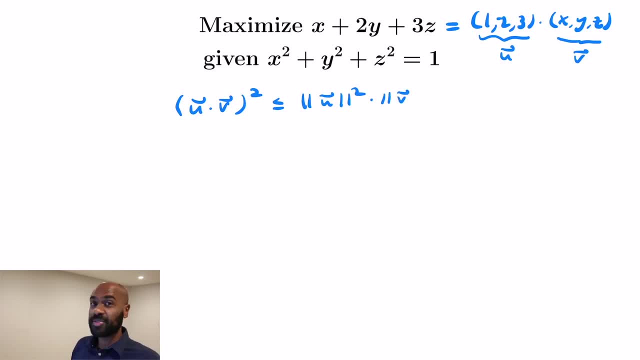 And v squared is less than or equal to the square of the length of u times the square of the length of v, Okay, and we can fill some of this in. so u dot v by construction- is the square of the thing we're trying to maximize. is x squared, x plus 2y plus 3z, all squared, and we're saying here that it's less. 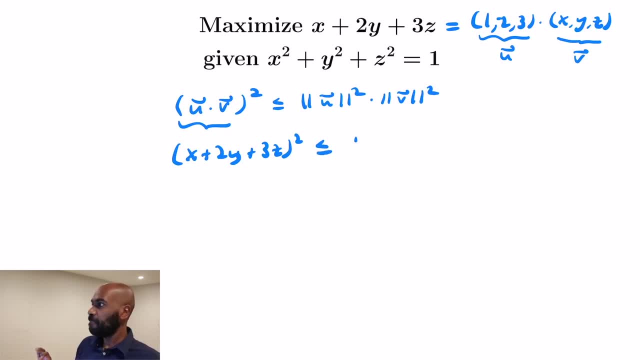 than or equal to the square of the length of u, which is 1 squared plus 2 squared plus 3 squared all times, the square of the length of the vector v, which is x squared plus y squared plus z squared. Okay, so this is great because we have 14 as one quantity, and then x squared plus y squared plus. 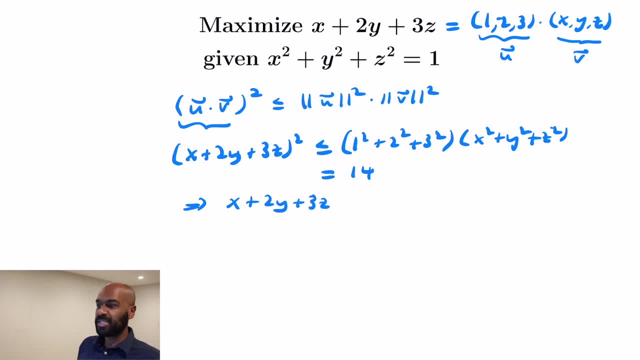 z squared is 1 in our situation. So x plus 2y plus 3z is less than or equal to the square root of 14.. And we actually know this square root of 14 can be achieved. Equality is achieved when the vectors u and v themselves are equal. 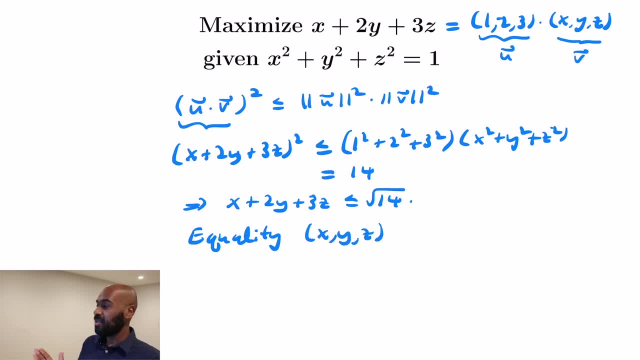 They are parallel. Okay, so that means the vector x, y, z is parallel to the vector 1, 2, 3.. So if you look at the components of x y z, we can relate them all to x. y is going to be 2x, z is going to be 3x. 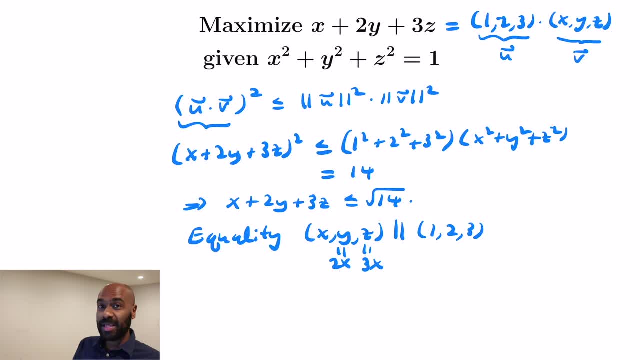 Okay, and then we can actually figure out what that vector has to be, because of the fact that the sum of the squares are constrained to be 1.. So we can get x squared plus the quantity 2x squared plus the quantity 3x squared is all 1.. 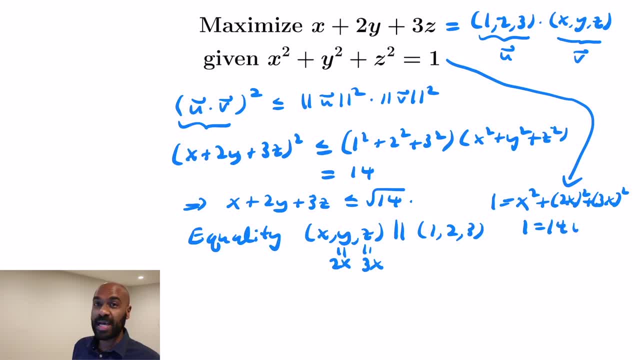 Okay, and then that tells us then that 1 is 14 times x squared, which means that x is either positive or negative, 1 divided by the square root of 14.. Great, so then the vector itself, the vector x, y, z, we're going to know all the components of. 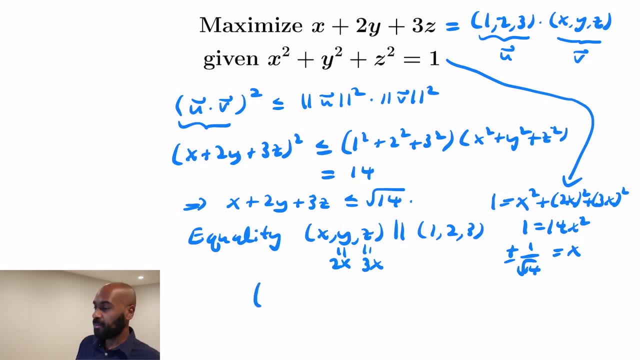 for when equality holds. So we get 1 over root 14,, 2 over root 14,, 3 over root 14 or the same vector with negatives in all of the components. So this is where our maximum in our problem is actually achieved. 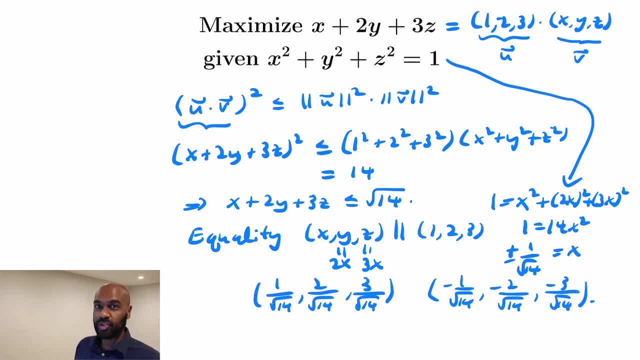 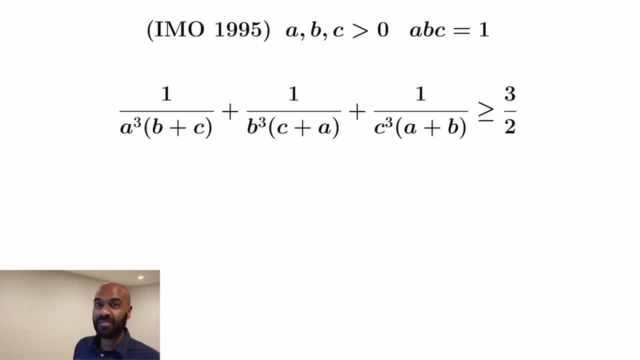 Cool. so a great application of Cauchy-Schwartz. Now let's go ahead and use the Cauchy-Schwartz inequality to solve a problem from the 1995 interview. So this problem says you have three real numbers- a, b, c- and they're all positive. 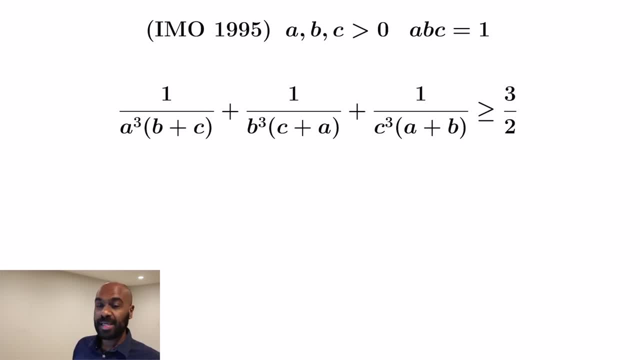 and their product is 1, and it asks to prove that the quantity 1 divided by a cubed plus b, c plus the same thing done cyclically over all the variables, is greater than equal to three halves. So it doesn't look like at face value that we can actually use the Cauchy-Schwartz inequality here. 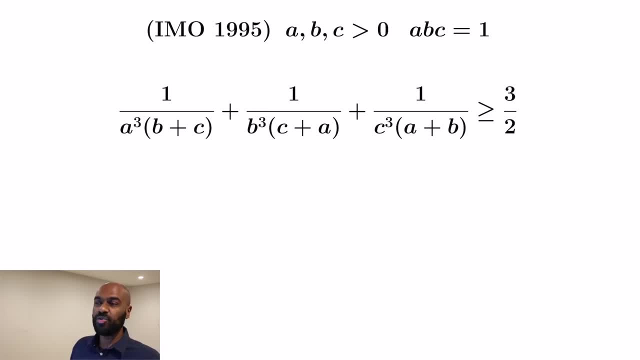 So we're going to do is use this problem to solve the Cauchy-Schwartz inequality. So we're going to use this problem as a way to suggest a method to use the Cauchy-Schwartz inequality when it seems like it might not be useful. So we're going to underline the. 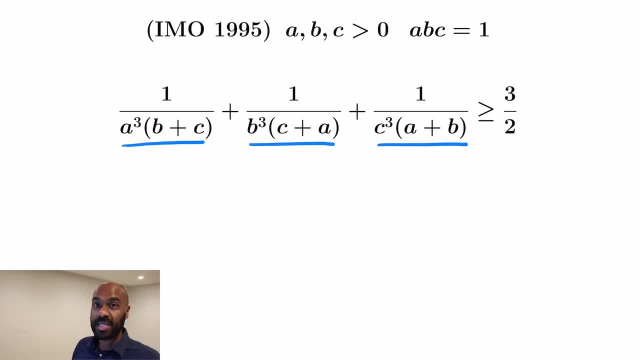 denominators here and think of them as pieces of vectors, like we did in the previous problem, And then use that together with Cauchy-Schwartz to get something involving an inequality like the type that we want. Now the question is, how do we do this? We have a lot of choices. 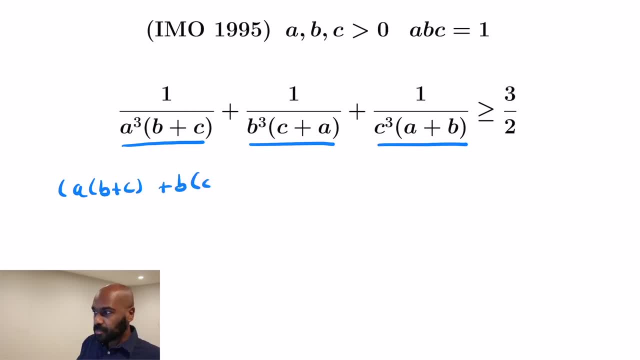 So what we're going to do in this particular case is think about those denominators as being parts of vectors and then create another vector. That vector is going to have as its components a times b plus c, b times c plus a, c times a plus b, And we're going to make these as squares. So we have 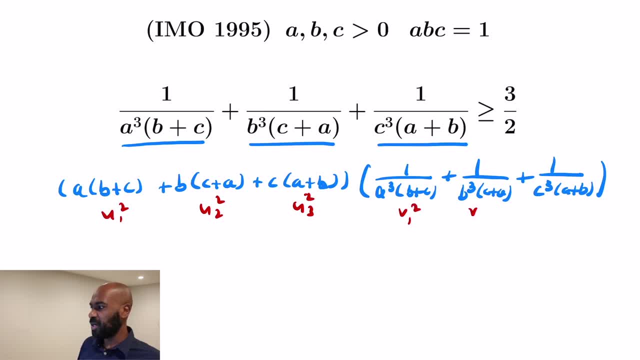 u1 squared, u2 squared, u3 squared, and then v1 squared, v2 squared, v3 squared- right over here. Okay, the advantage of doing this is now the whole point of Cauchy-Schwartz- is it relates the components of these vectors that we're dealing with. 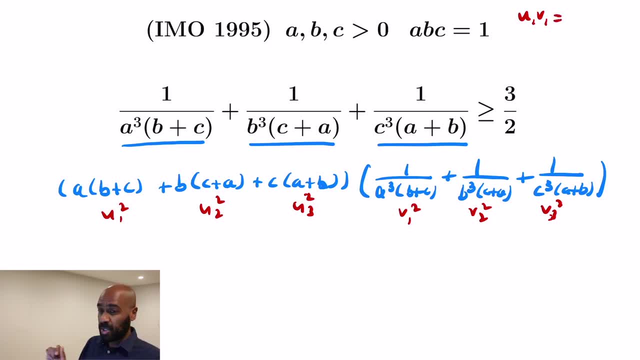 and takes the dot product of them, and that involves multiplying the corresponding matching coordinates And, in this case, introducing the factor, the ui's- that we have, we get that the product of u1 and v1 is 1 over a, the product of u2 and v2 is 1 over b and the product of u3 and 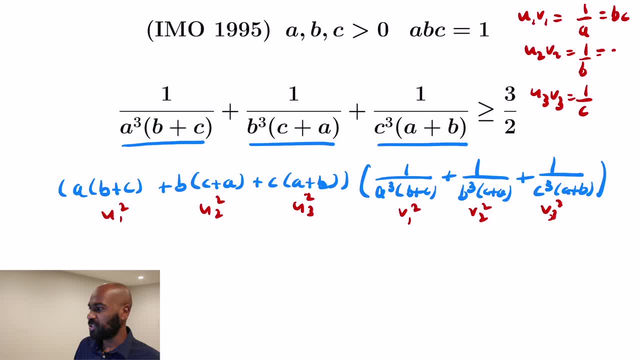 v3 is 1 over c, So they're constructed to do this interesting product. that makes things simpler. And then, because abc is 1, we get that 1 over a is bc, 1 over b is ac and 1 over c is ba. 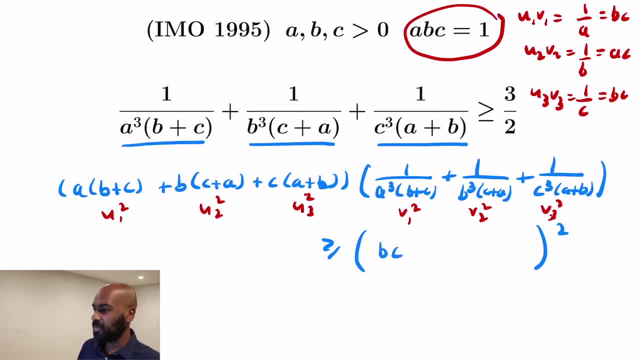 All right, so this quantity then is going to be greater than or equal to by Cauchy-Schwartz: bc plus ac plus bc all, or let's just say ba all squared. Okay, so all together, then, we have our product. we notice that this thing actually is related to the sum of the squares of 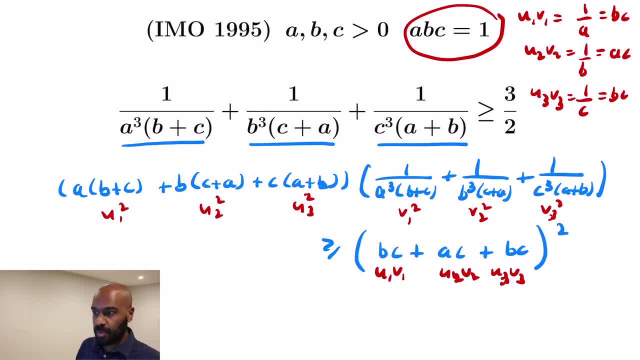 the components of the ui's. If you look at the sum of the components squares of the components of the ui's, it's actually a constant factor times the quantity bc plus ac plus ba. Again, that b, second bc, should be a ba there And that's going to help us because then we can divide out and then see a. 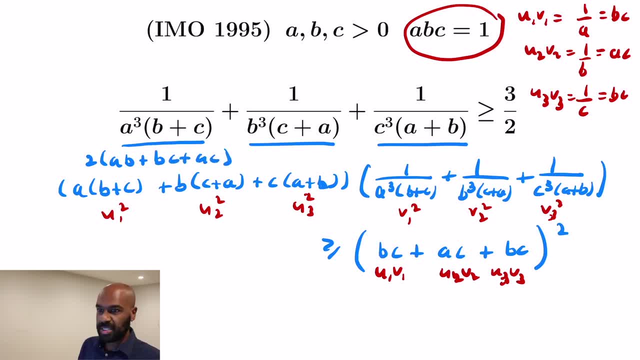 relationship for a lower bound for the quantity that we're dealing with. So bc is 2 times ab plus bc plus ac. So this quantity that we started off with will have a lower bound now by dividing by this quantity we just underlined right up here. 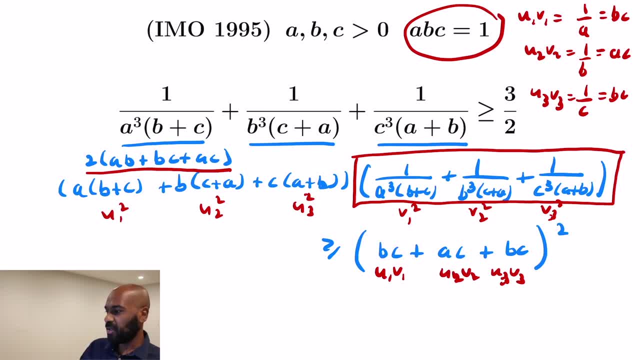 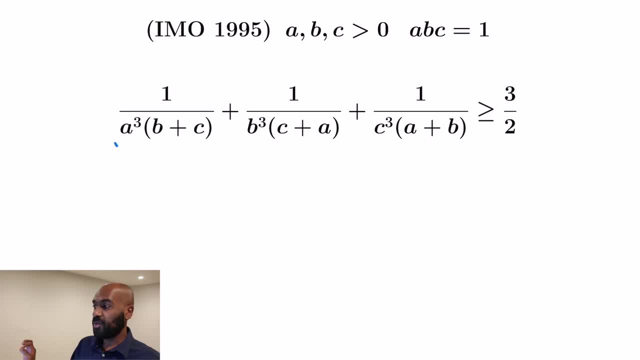 Okay, so let's go ahead and do that. It's one copy of the thing that we're squaring, so we'll be left with the thing that we were squaring to begin with, all divided by 2 as a lower bound for the actual expression that we were dealing with in our problem. So this is going to be greater.